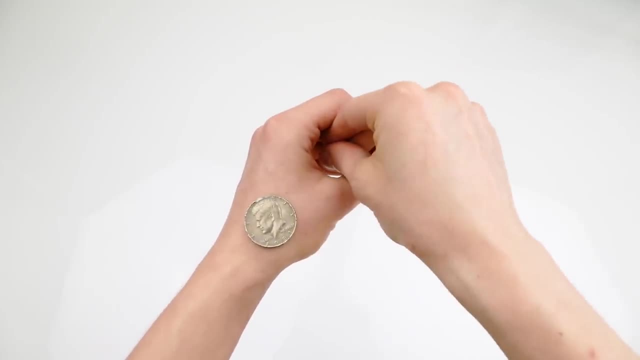 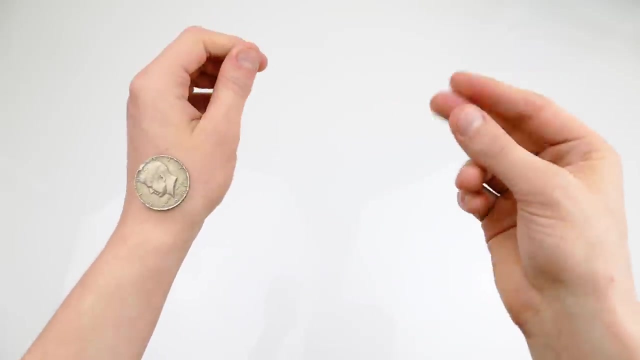 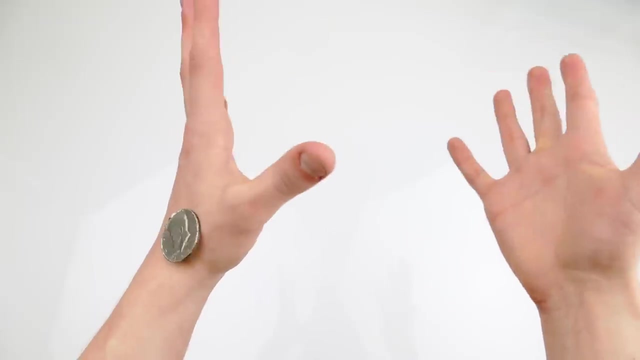 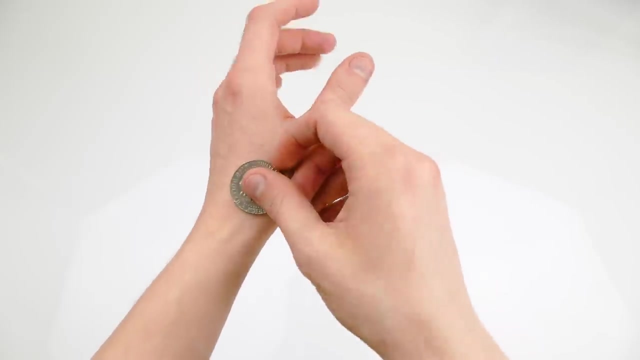 different Dirty Yeah. You act like you are holding the coin inside by, you know, squeezing the fingers back together So it looks like you placed the coin. You place it in like that, Snap your fingers and it vanishes. Or, if you want, you can open your fingers slowly, like that, and show that it's fully vanished And basically the coin is really loose. It can fall off any point. If you are sweaty it will help, but it can fall off any point. So you go and grab a coin. 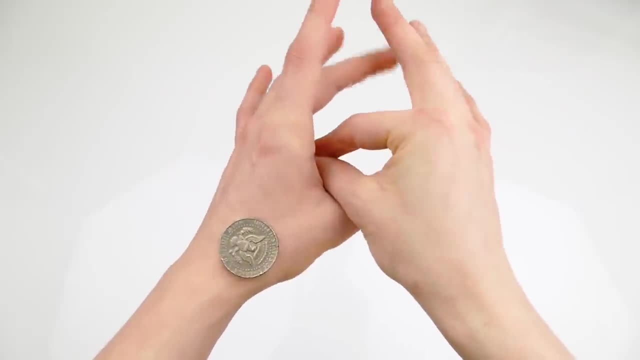 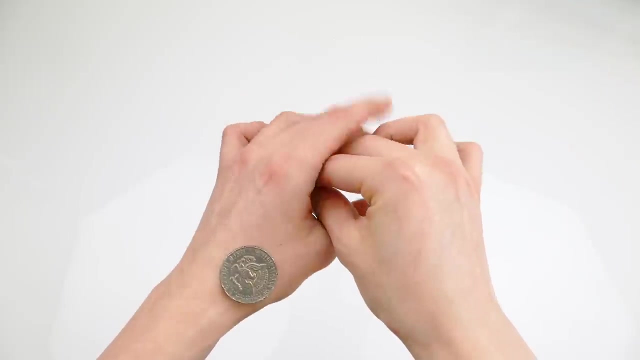 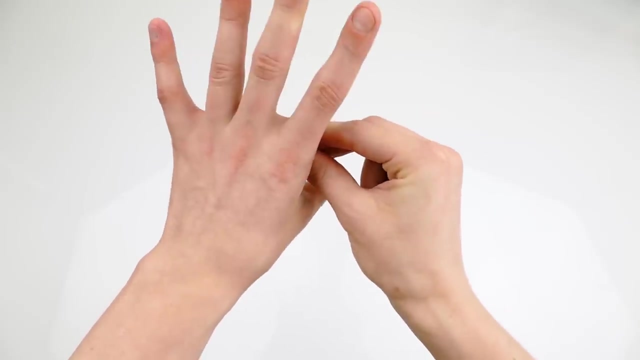 Out of thin air. You know, you grab it like this, You place it down here once again with all these three fingers, You grab it with the index finger and thumb, You place it down And then you take the coin like that, And when you're going to reproduce it, then what I like to do is I like to open my fingers slowly and like that. It looks quite visual and quite magical if you open your fingers like this. 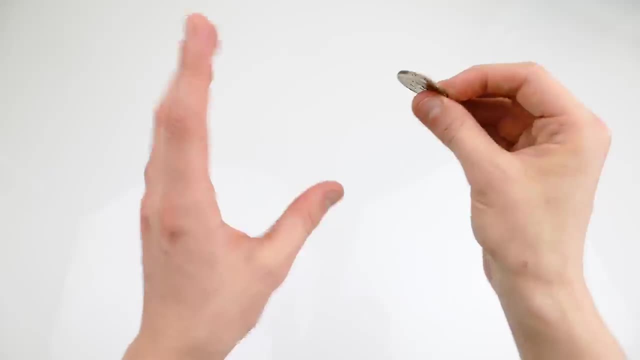 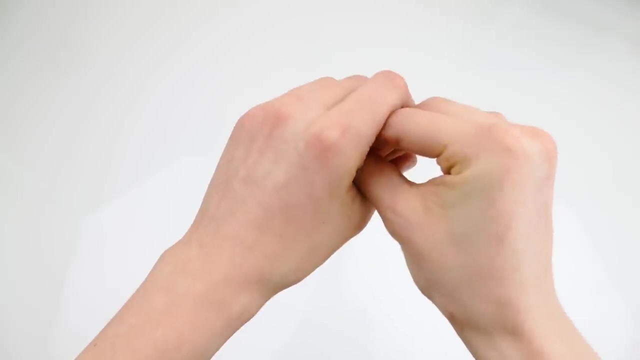 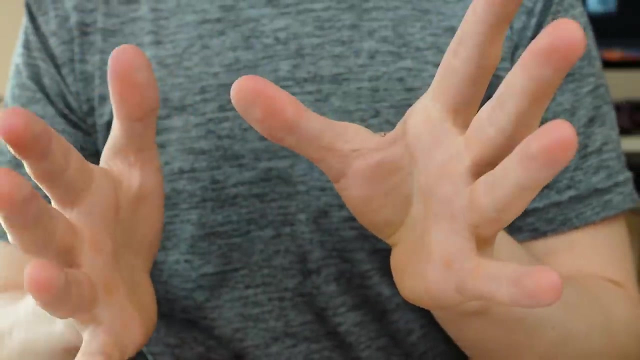 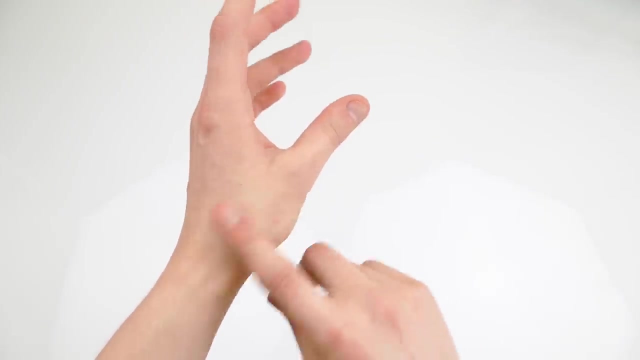 And then boom, Just like that Looks actually quite cool And in speed. this way would look something like that: Grab a coin, Take it there, Grab it like this, And it reappears inside the hand. That is the first way. The second way of doing this looks like this: What you're going to do is you are going to lick this part of your hand. You're going to make sure that there is a little bit of moisture on top, So you know it's a little bit sticky. Once you have licked it, you are going to 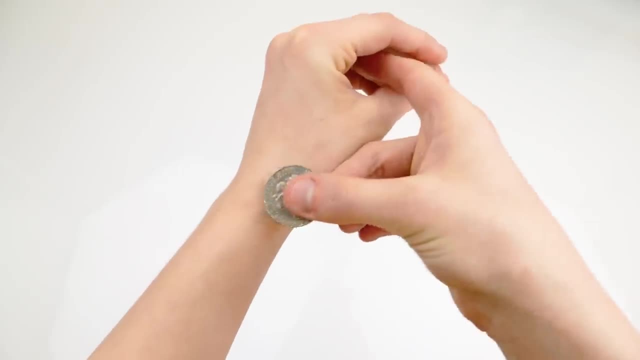 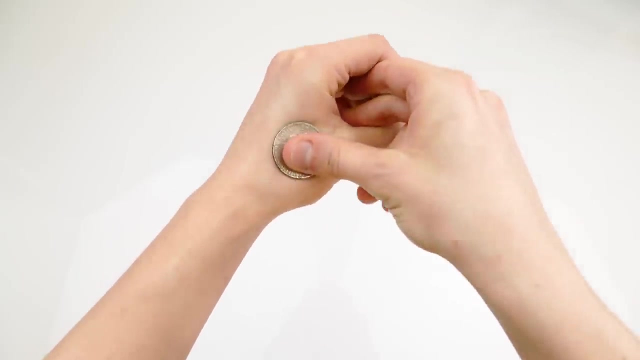 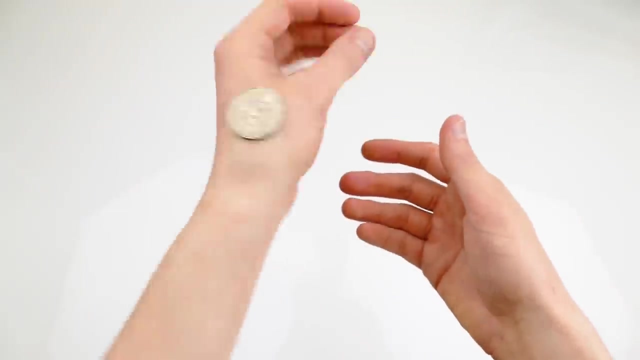 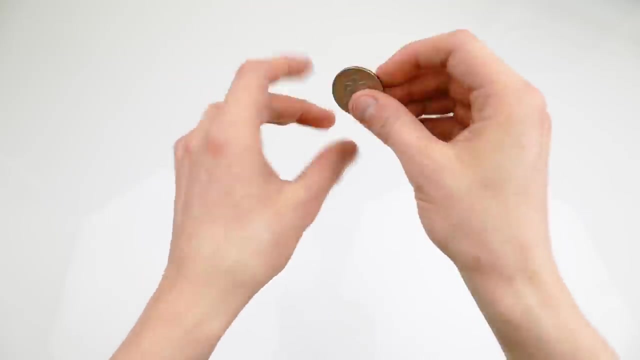 do the exact same thing, but this time, instead of placing it down here far away from the hand, you are going to place it near the top of the hand and you are going to squeeze a little bit. Just squeeze a little bit And, as you can see, look how the coin is sticking to the hand. This is brilliant. Look at that. There are a few similar coin vanishes to this. There is a coin vanish that someone showed me before where you do this and then you use the skin. 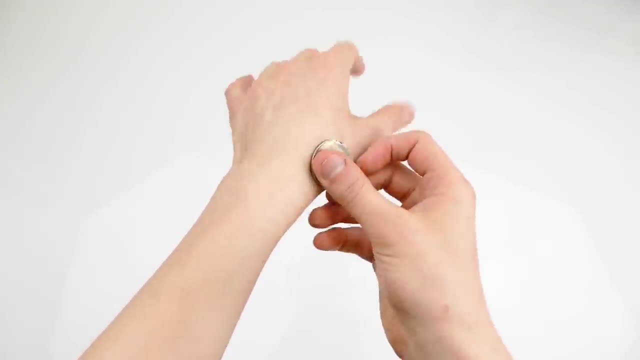 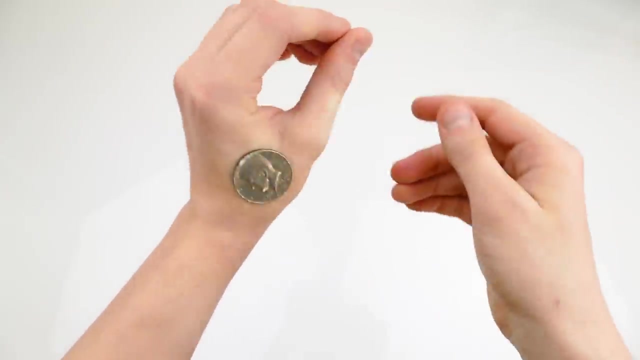 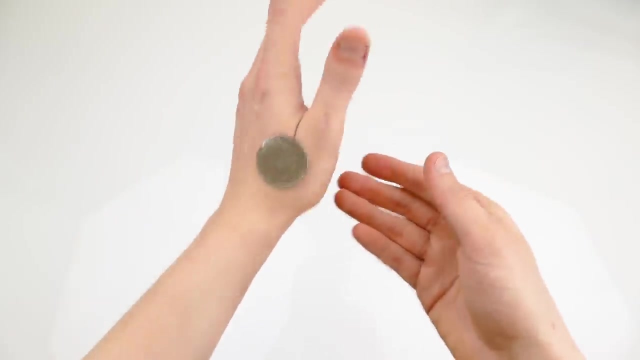 To hold the coin like that, And you know I never really liked it because I can't do it. So in my opinion this works way, way better. And then you know, when you have pressed on the coin and made it vanish, you can feel how sticky it is, And if you want it to stick less, then you can move your. 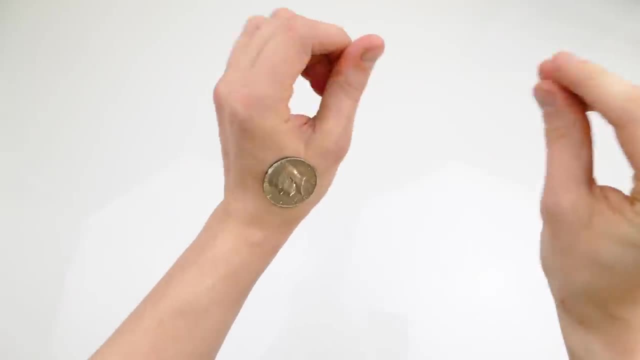 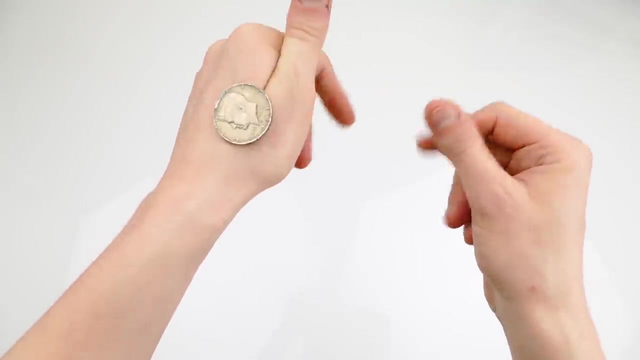 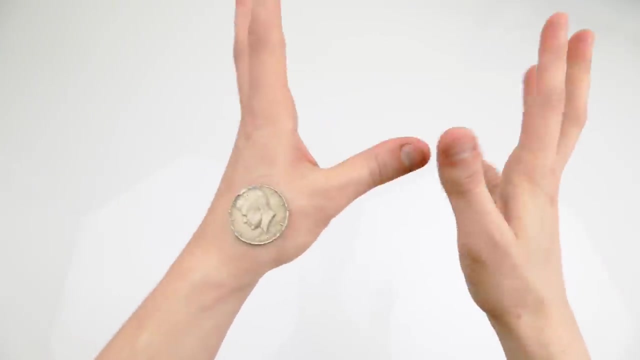 hand like that. So you know, you place it like this, Vanish it. And then you can move the hands like this, And then when you move it like this with your thumb, you are separating the coin from the hand. So once you press, make it vanish, it is sticky. And then if you do this and say, boom it. 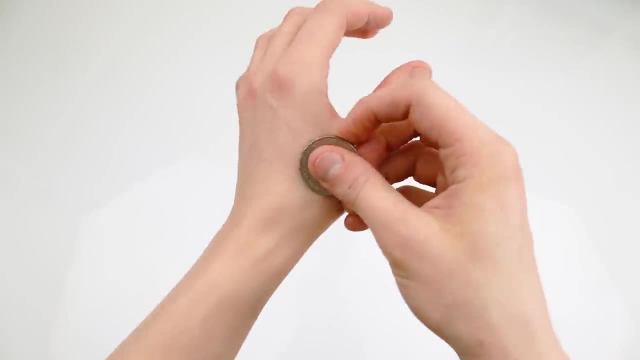 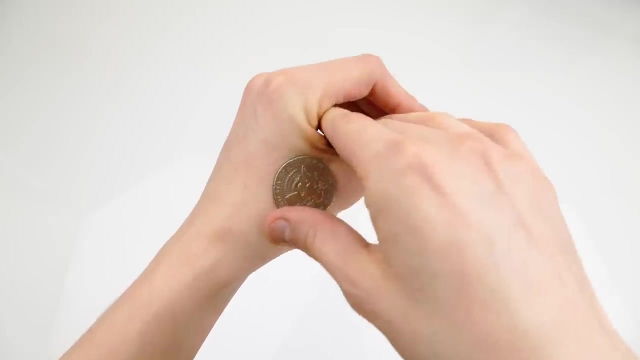 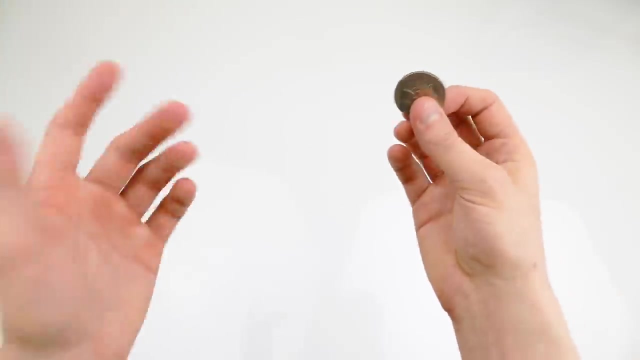 vanishes. Now the coin is less sticky and can easier fall off. Once you are in this position- less sticky, right now- you grab a coin like that, Take it and then make it reappear once again. This is actually quite cool, You know. if you want, you can, you know, make it vanish And then you can take it. 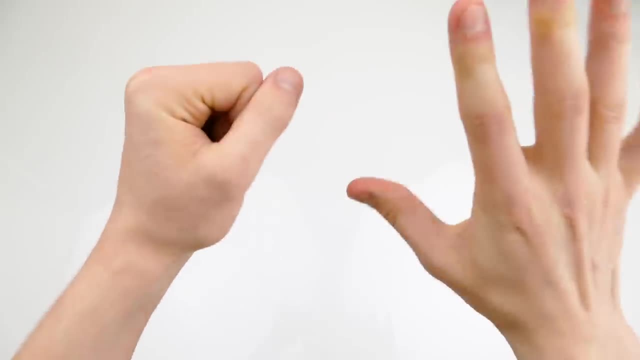 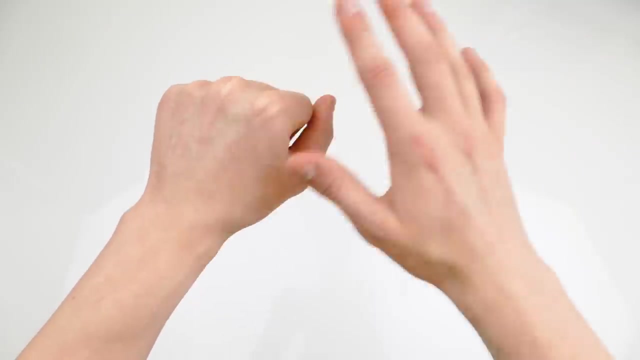 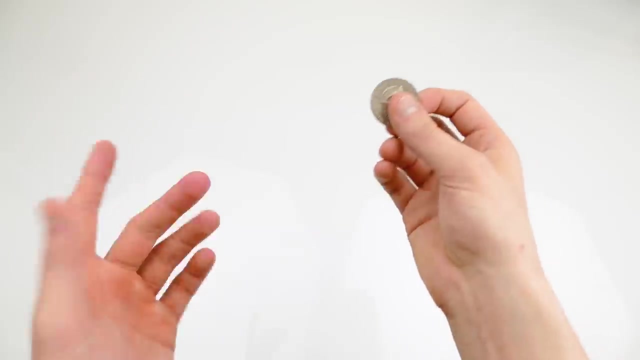 Make it reappear. But instead of opening the hand, you can remove the hand And then you are so clean you can show everything You know. you can show from every side right now that there's nothing on your hand. Then you can snap your fingers and show that the coin reappeared And that looks. 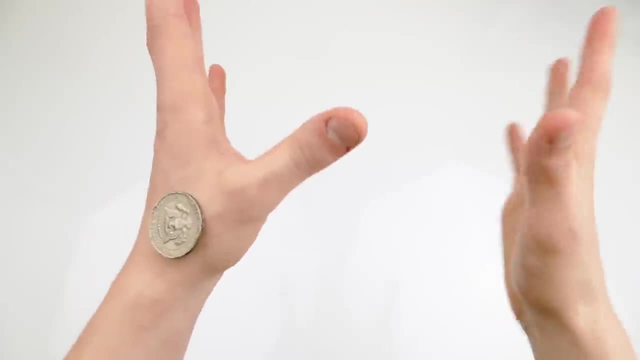 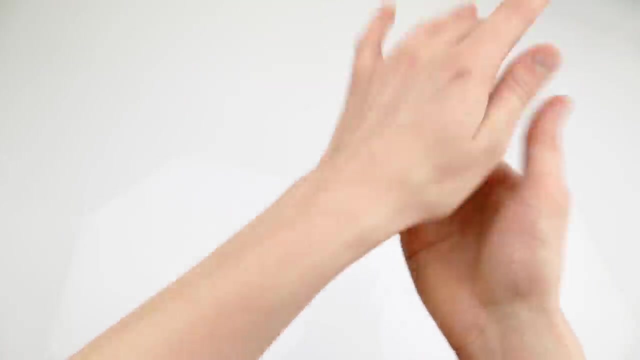 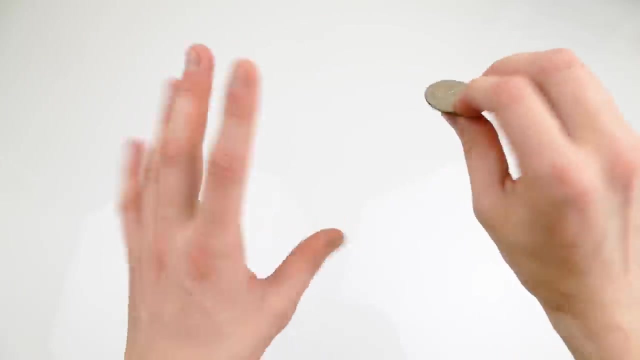 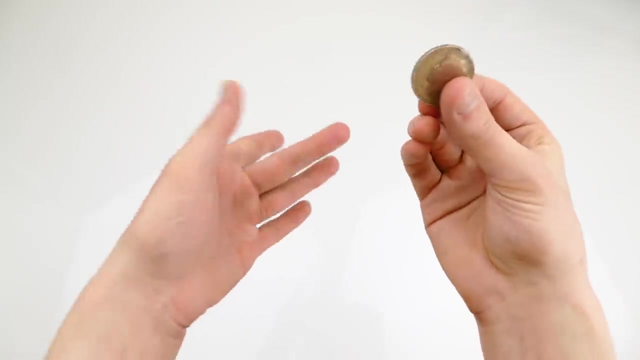 really really good, Something that you can do, And a lot of people do this And I think it's really cool. I think it's really cool. A lot of different magicians they have been, you know, doing this type of coin: vanish, Where you take it, place it And where you do something like that: Whatever you want to do, Vanish it And then boom, If that's something, then you can easily do it. So thank you for watching. I hope you enjoy this. I'm thinking about some tips that I can tell you, But I don't really have any tips. Let me do it slowly And you can follow along So slowly. it looks like this: 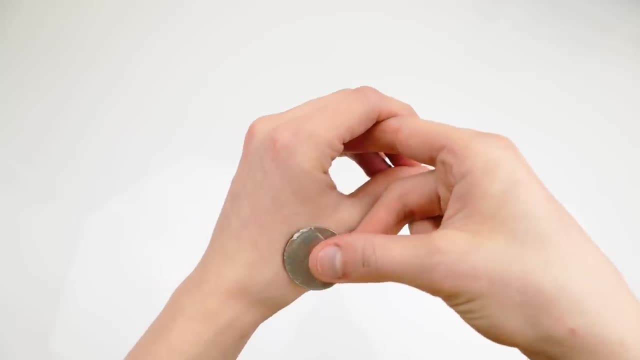 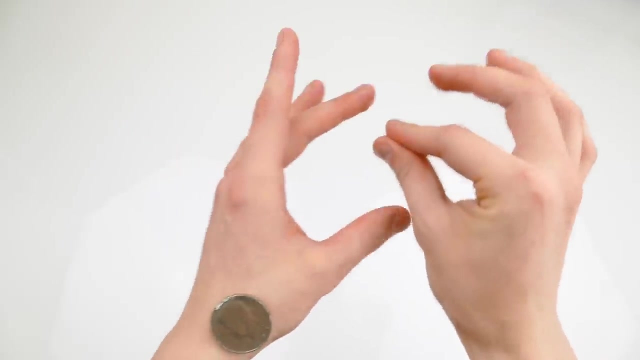 Great. Grab it, Place it on top Of the hand, Push my middle finger inside, My thumb inside And, you know, Make it vanish Whatever you want. And then grab a coin Like that, Pull this coin up And then boom. 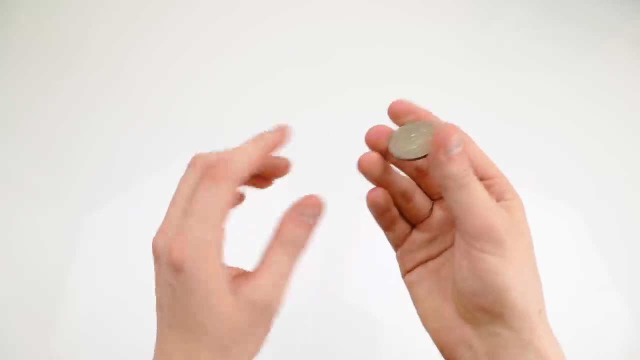 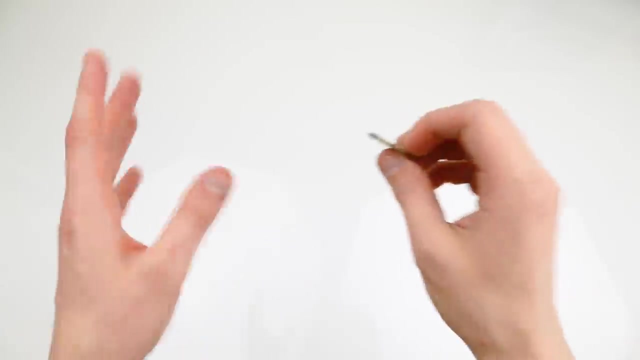 Just like that. So that is how it looks like. Hope you enjoy this video. There are so many different coin vanishes you can do. There is this coin Vanis, which I do have a tutorial on, and a lot of different coin vanises as well, if you want to check it out.